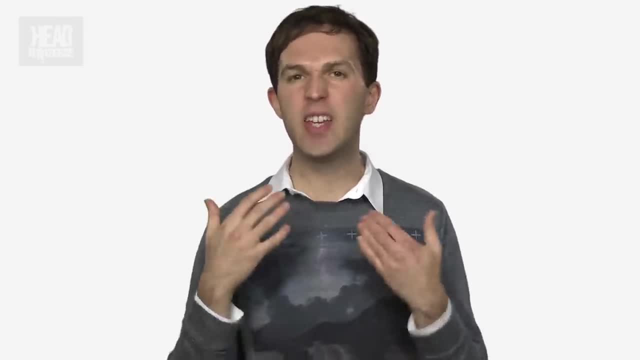 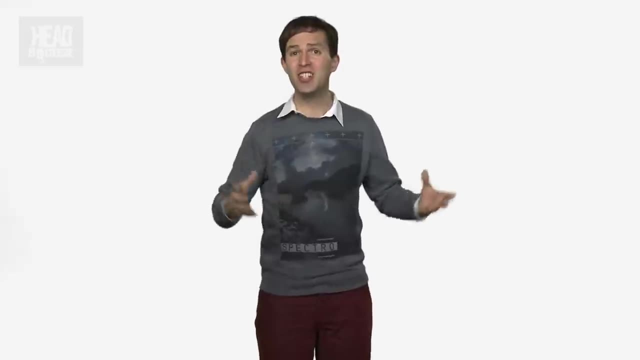 doesn't actually give you the full 3D experience. It gives you that sense of depth, but it doesn't give you what's called parallax. That means if you move your head around, the view doesn't actually change with a 3D movie. Now there is a way of doing this, and that's using holograms. 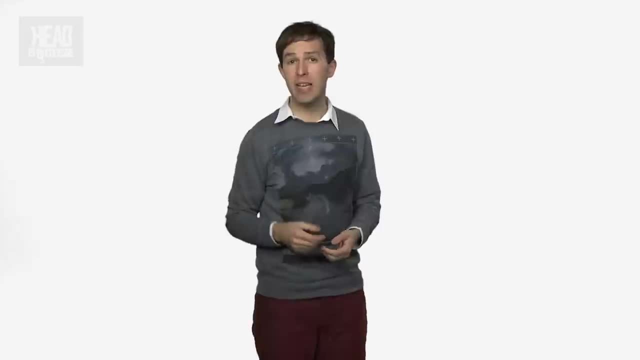 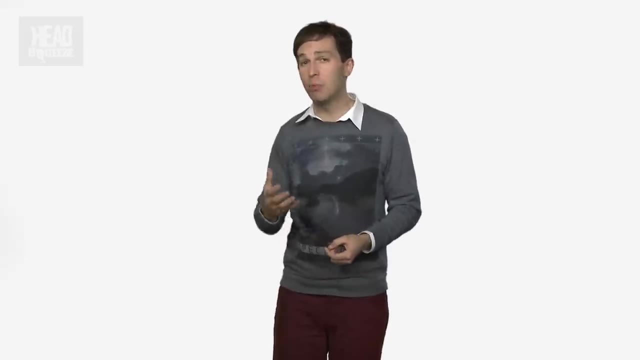 Holograms were actually invented in the 1940s by Dennis Gabor. It earned him the Nobel Prize in 1971, but it wasn't actually until the 60s that they started doing holograms with light. Previously it was with electrons, and that's because the laser hadn't been invented yet. So how does a hologram actually work? Well, if we go back to the beginning of the 20th century, there was a hologram that was made out of light and it was made out of electrons, And that's because the laser hadn't been invented yet. 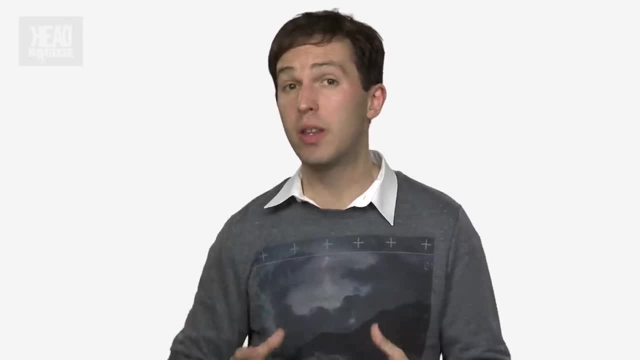 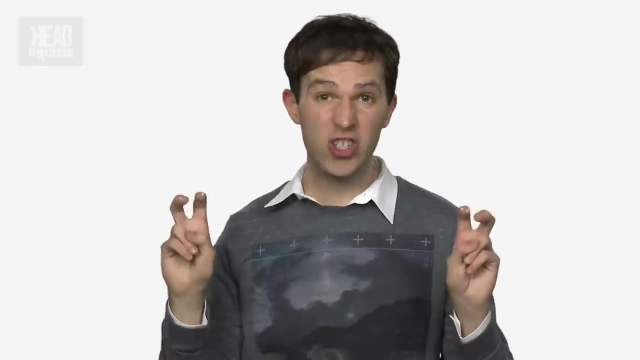 So let's go right back to basics and think of a photograph to start with. How do you make one of those? Well, you have an object, the subject of your photograph, and light bounces or scatters off of it. Now, that light's probably from the sun or the flash in your camera. 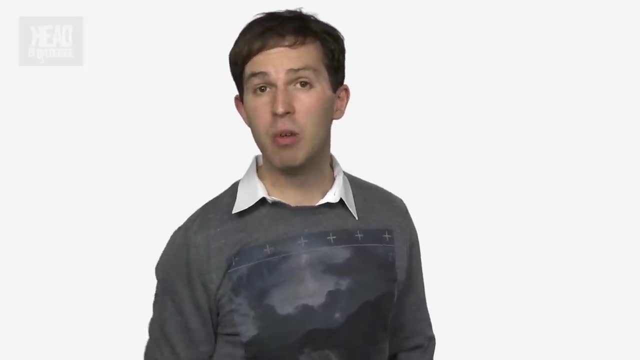 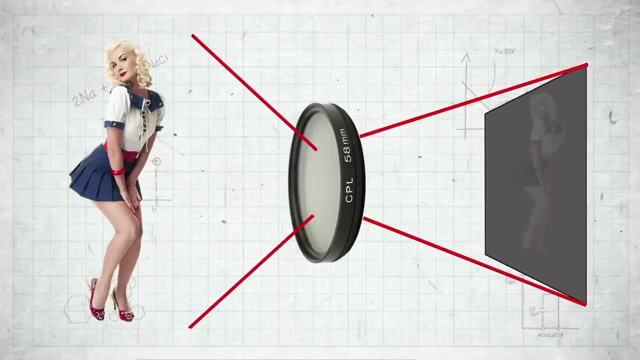 Now that scattered light is then going to go through a lens in your camera and then hit the CCD. if you've got a digital one, or if you're old school- a photographic plate, Then encoded on that photographic plate, you have the intensity. 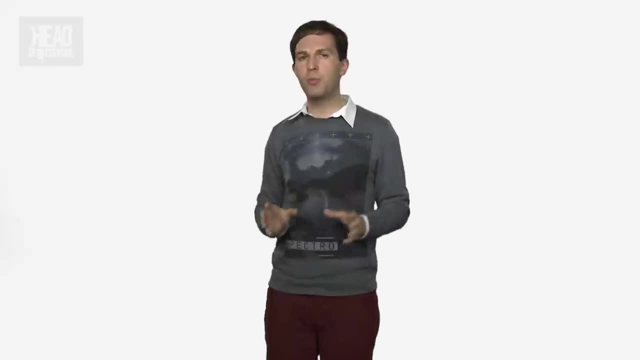 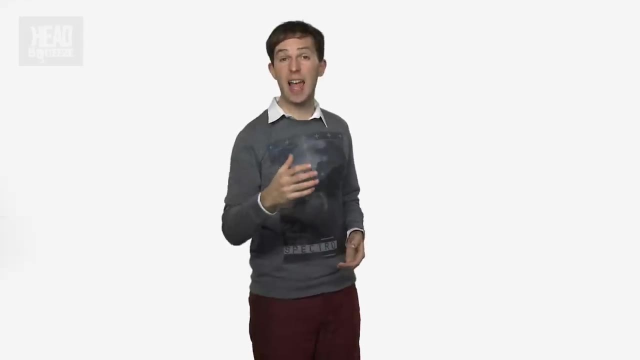 of the light that bounced off of that object. Now there's actually one property of the light that we have missed. It's called the phase, and that's actually related to the distance the light has traveled from the object. We can't capture that in a photograph, but in a hologram you can. 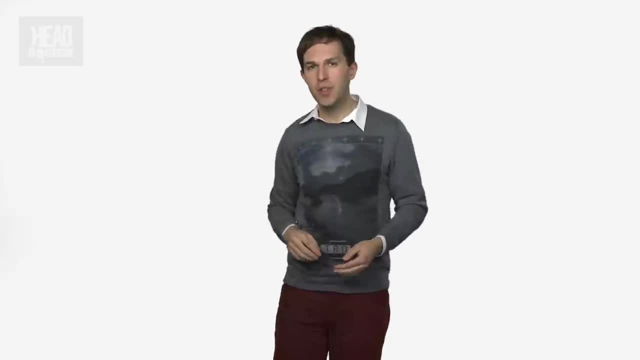 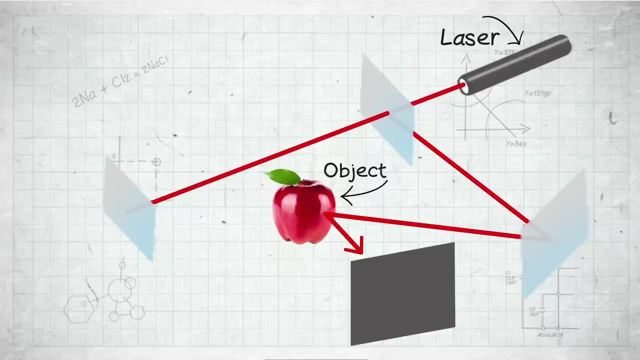 because the setup is slightly different. If you start off with a laser, you take the laser beam and you split it into two: One of those we're going to use as a reference beam and the second one we're going to bounce off of. 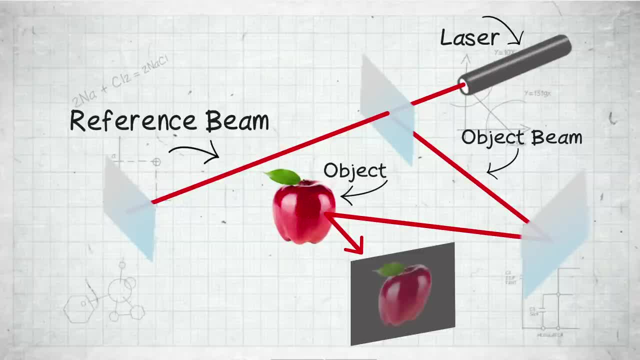 So, just like with a photograph, you have light bouncing off an object which then hits a photographic plate- Great. What you need to do now- which is different from a photograph- is reflect that reference beam into that plate. What that's going to give. 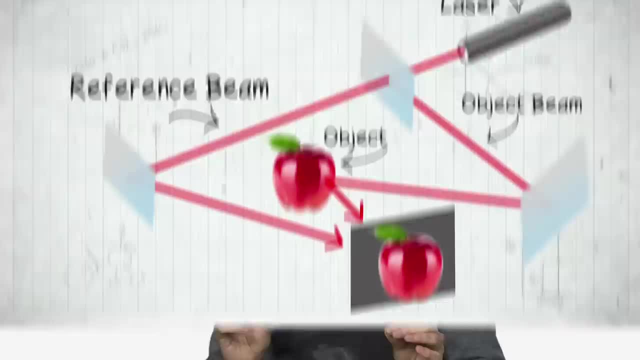 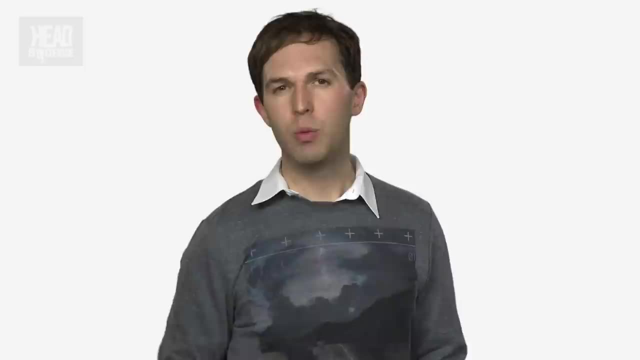 you is an interference pattern between the two beams, and that is what allows you to capture the phase. And there you go: You've made a hologram. Except if you look at it with your naked eye, it's not going to look like what you expect, because what you need to take